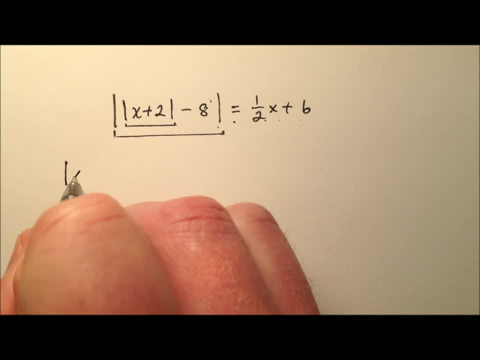 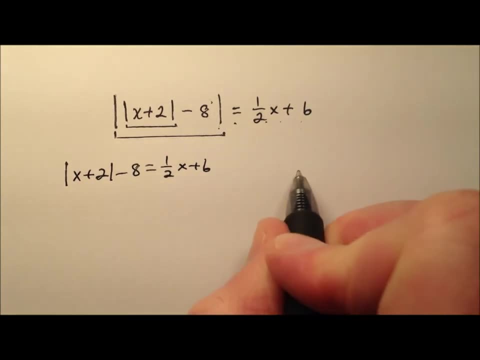 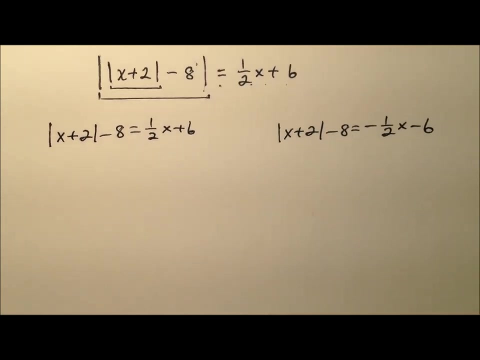 we take the positive and the negative. So we're going to say the absolute value of x plus 2 minus 8 equals positive 1 half x plus 6.. So we have this absolute value expression equal to 1 half x plus 6, and the absolute value of x plus 2 minus 8 equals negative 1 half x minus 6.. So here I've. 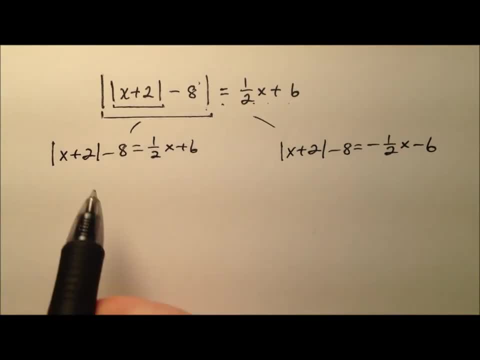 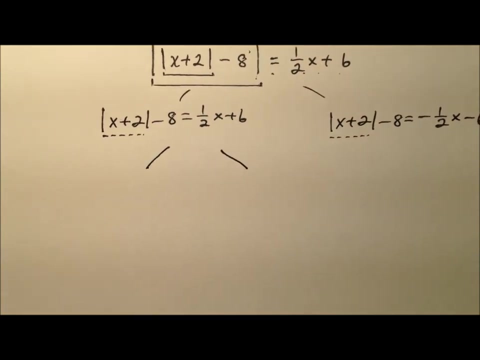 split it up into my two separate equations and you'll notice again I still have absolute value expressions, so I'll need to split it up again into two more. So ultimately I'll have four equations to solve. So let's go ahead and make this one down into two separate ones, So we'll 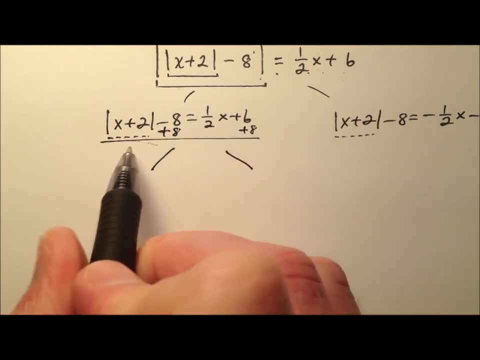 add 8 to the absolute value expression and then we'll split it up again into two more. So we'll add 8 to the absolute value expression and then we'll split it up again into two more. So we'll first, and I'll end up with the absolute value of x plus 2 on the left side equals 1 half x plus 14. 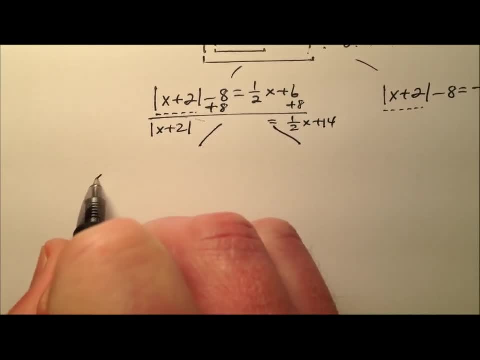 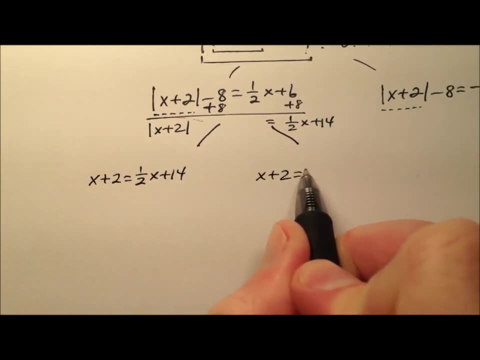 on the right side. So when we split this up, it'll be: x plus 2 equals 1 half x plus 14, and x plus 2 equals negative 1 half x minus 14.. So we'll go ahead and solve these two first, and then we'll. 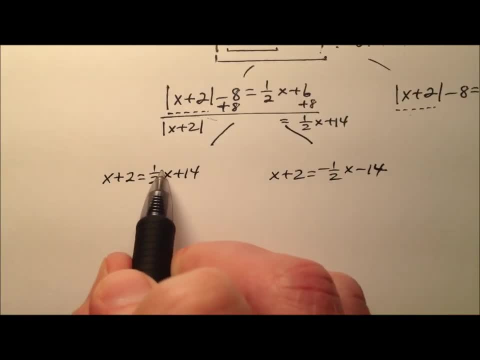 go back and deal with this other equation. So I can subtract 1 half x, so 1 minus 1 half will give me the 1 half x, and then 14 minus 2 is 12, so in this case x will be 24.. 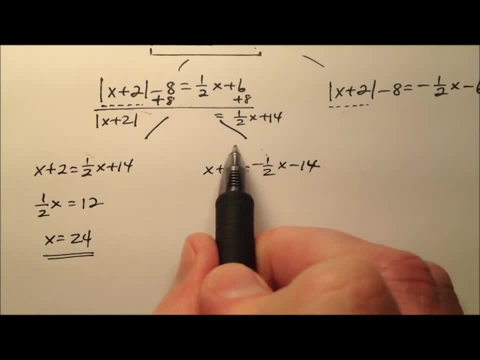 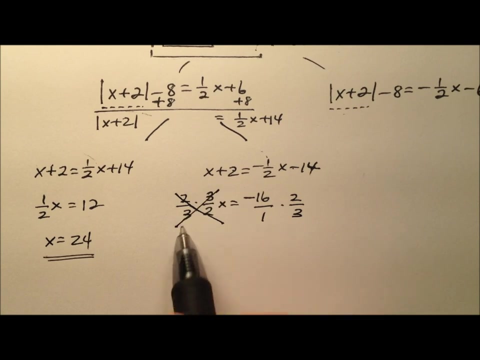 Alright. well, how about? here? I can add 1 half x, so I'll have 3 halves x equals, and then negative 14 minus 2 is negative 16, and so I'm going to go through and multiply both sides by 2 thirds. so the 2 halves x equals 1 half x plus 14.. 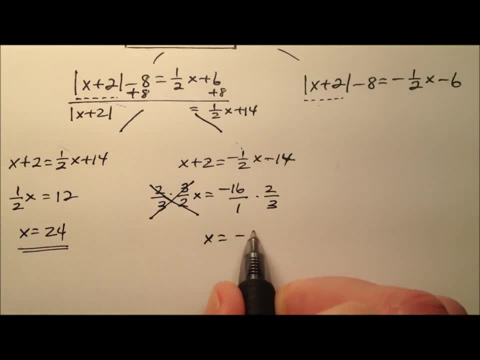 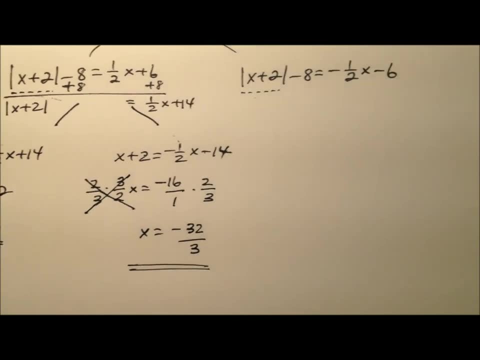 2's and the 3's both cancel. So x actually equals what Negative 32 thirds? Okay, so there's that possible solution. So we need to do the same thing with this one. So when I add 8 to both sides, 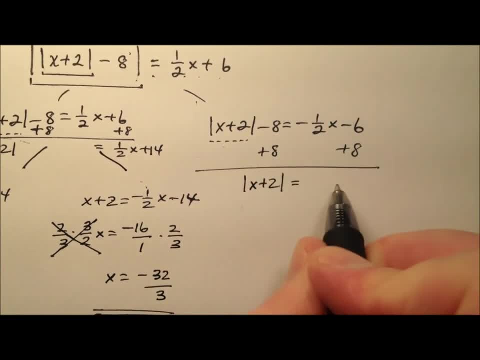 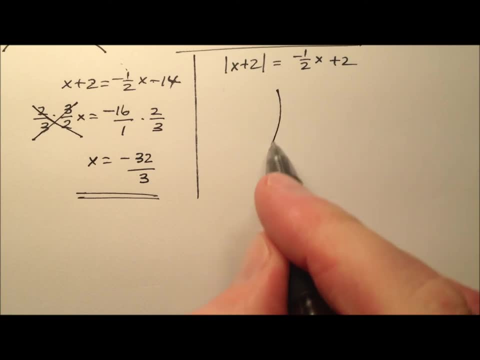 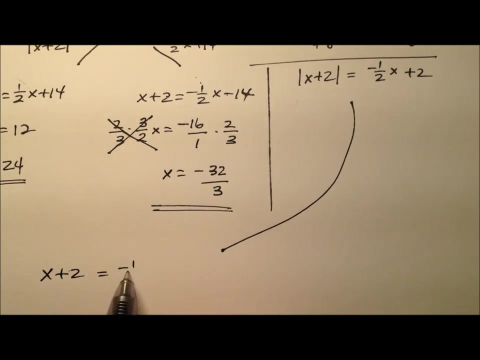 I have the absolute value of x plus 2 on the left and negative 1 half x plus 2 on the right. So I'm going to go ahead and kind of bring that down here and divide it into two separate equations. I have, when x plus 2 equals the negative 1 half x plus 2, and the x plus 2 equals positive 1 half x. 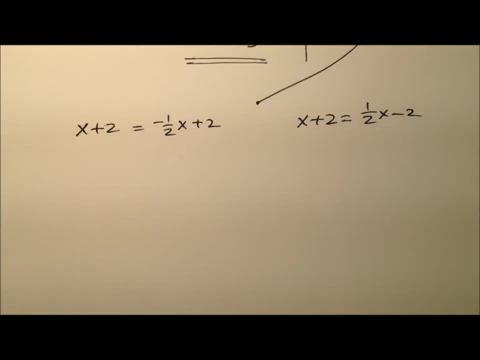 minus 2.. So there, I've gone ahead and split it up, So let's solve both of these. So when I add 1 half x, I get 3 halves x equals, and 2 minus 2 is 0.. So this critter is x equals 0.. 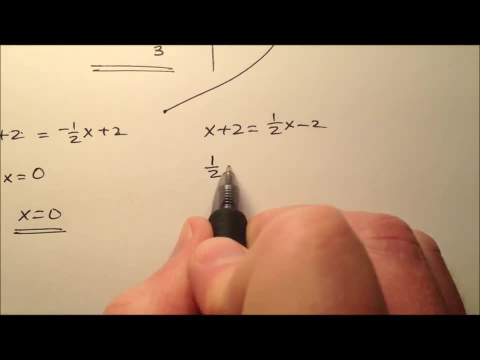 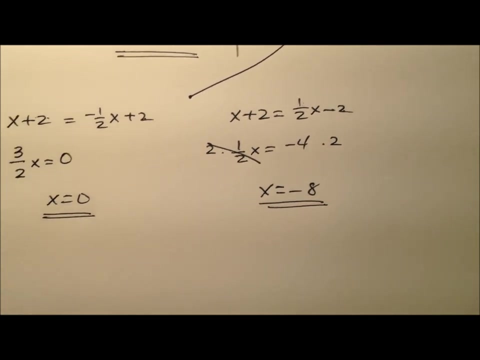 And this last one, I'm going to subtract the 1 half x, So I have: 1 half x equals negative 2 minus 2 is negative 4.. So when I multiply both sides by 2, x equals negative 8.. Okay, well, now I have four potential solutions, So let's go ahead and write. 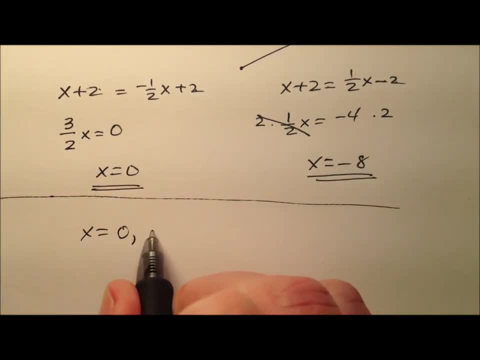 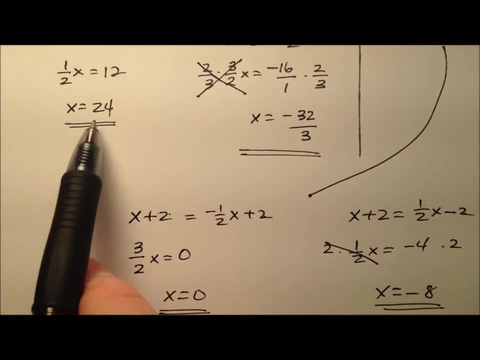 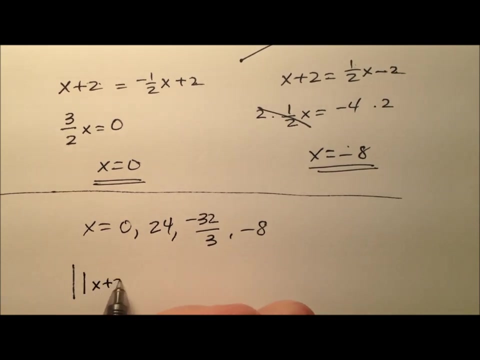 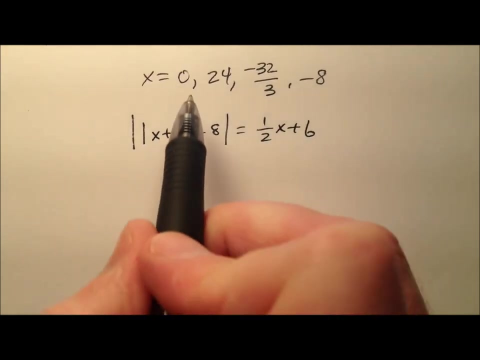 them all out here. I have x equals 0, 24, negative 32 thirds and negative 8.. And those are the four I found from solving each of these equations. Now I'm going to go ahead and rewrite my original equation and I'm going to solve and just see which of these work We'll start with: 0. That. 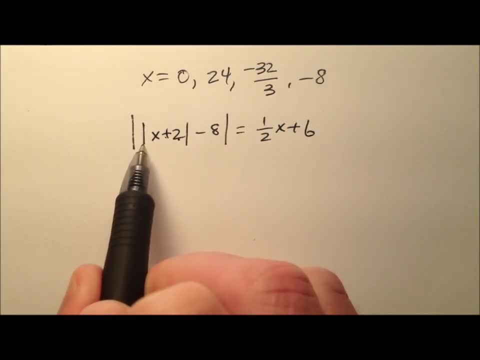 seems pretty easy: 0 plus 2 is 2.. The absolute value of 2 is well, 2. And 2 minus 8 is negative, 6. And the absolute value of negative 6 is positive 6.. So when x equals 0,, I have 2 minus 8.. And then, when x equals 0,, I have 2 plus 2.. And then, when x equals 2, I have 2 minus 8.. And then, when x equals 2, I have 2 minus 8.. And then, when x equals 2,. 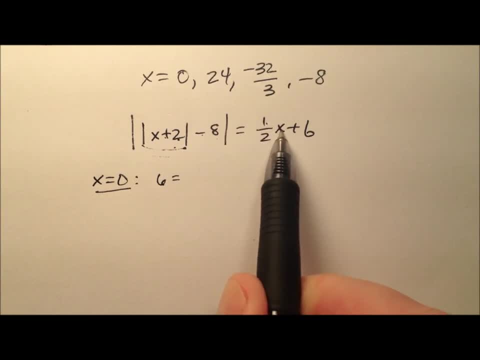 6 on the left side and 1 half times 0 is 0 plus 6.. Okay, so x equals 0 works, So let's try 24.. So 24 plus 2 is 26. Absolute value is positive 26. Minus 8 is: 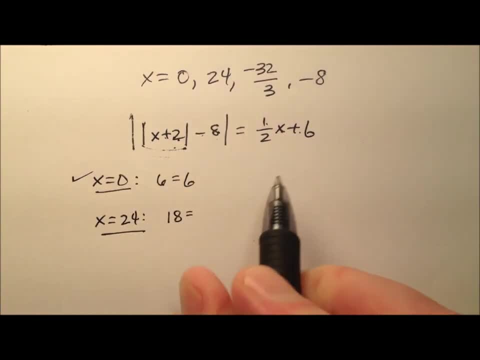 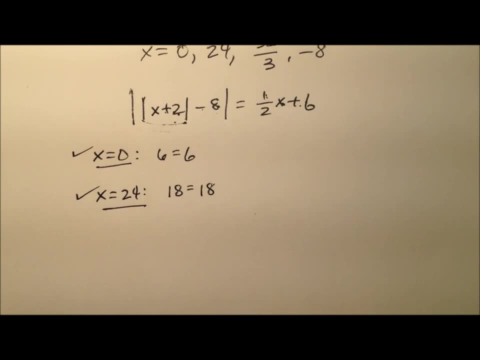 going to be 18.. Absolute value is 18.. So half of 24 is 12.. 12 plus 6 is 18.. Okay, that one works as well. Okay, so let's move on to negative 32 thirds. Okay so negative 32 thirds, and I can almost stop right here. Let's go. 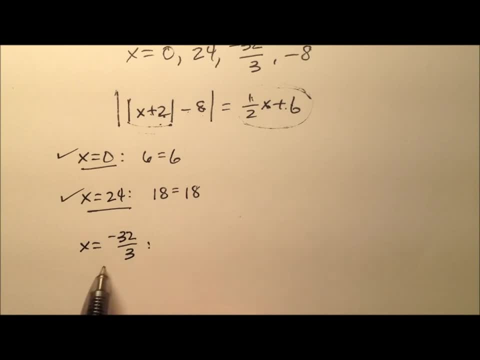 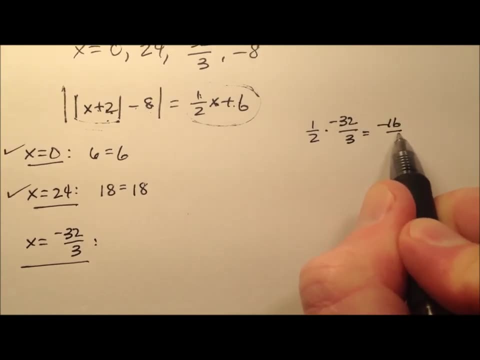 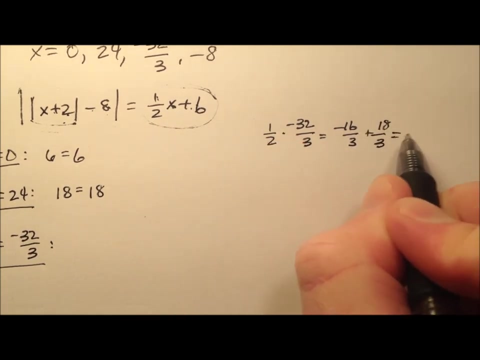 ahead and do the right side first. So 1 half times negative 32 thirds equals negative 16 thirds. and then when I add 8, I'll be adding. sorry, I'm adding 6.. I'm adding 18 thirds, which is 2 thirds. Okay, so the right side is 2. 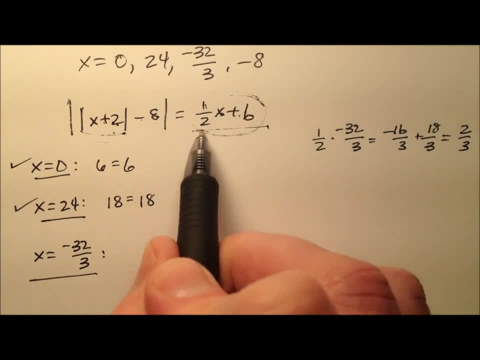 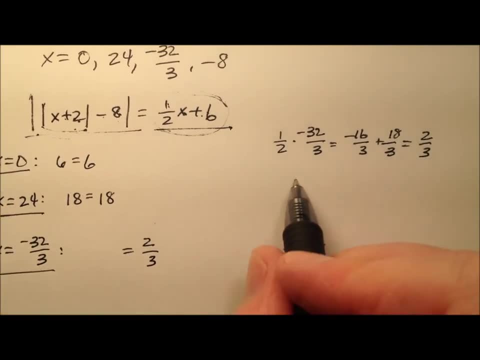 thirds. The reason I did the right side first is because if this came out to be negative, there was no reason to do the left side. Okay, so let's go ahead and do that left side then. So we have x plus 2.. So negative: 32 thirds plus 2.. So it's. 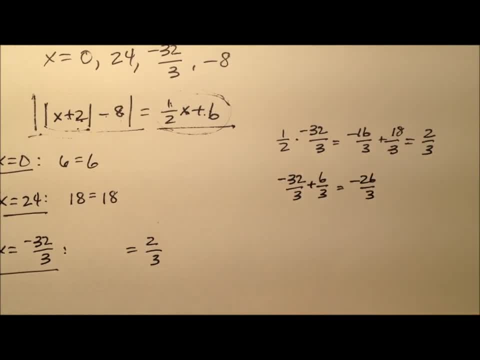 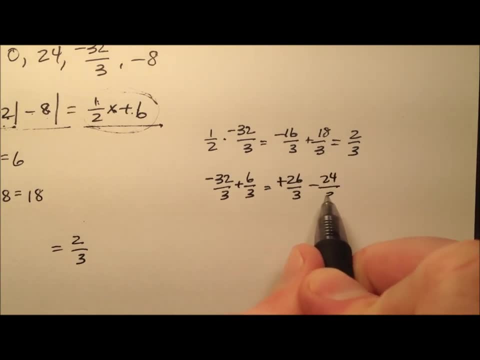 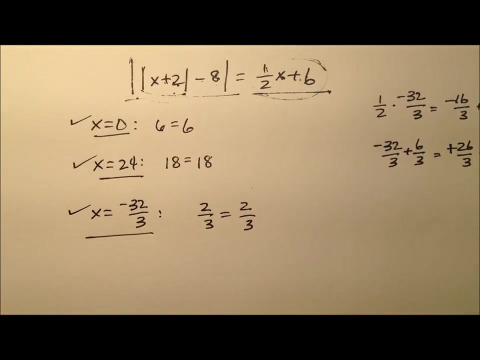 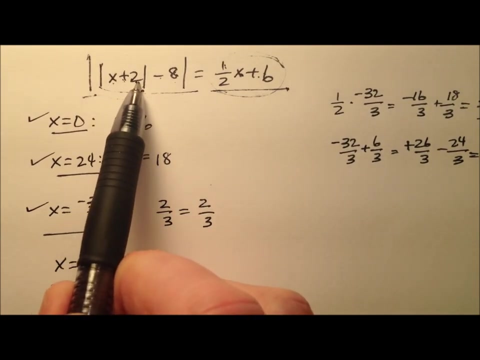 plus 6.. So negative 26 thirds. The absolute value of that makes it positive: 26 thirds Minus 8.. So that's minus 24 thirds is 2 thirds. Alright, so that works as well. And our last one is: x equals negative 8.. So negative 8 plus 2 is negative 6.. The 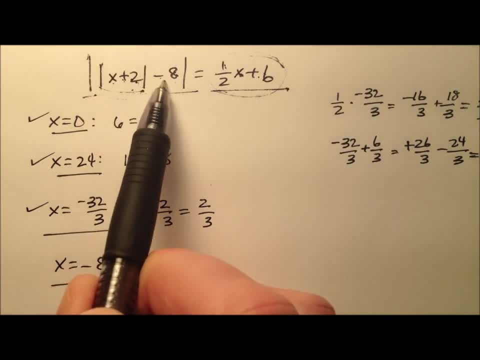 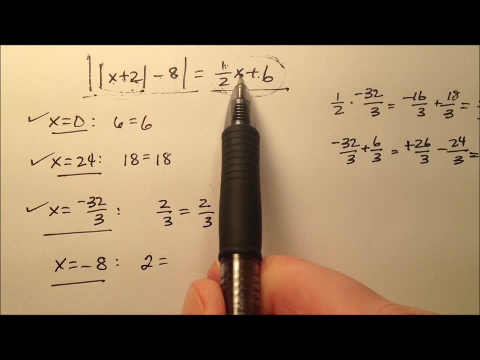 absolute value of that is going to be positive: 6. And 6 minus 8 is negative: 2. Absolute value of that is 2.. Alright well, 1 half times negative. 8 is negative. 4 plus 6 is 2.. 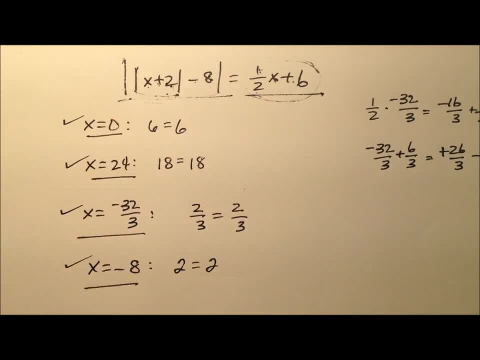 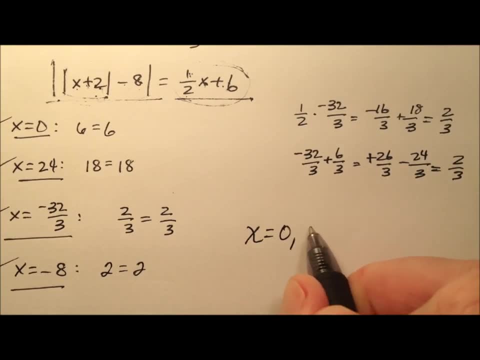 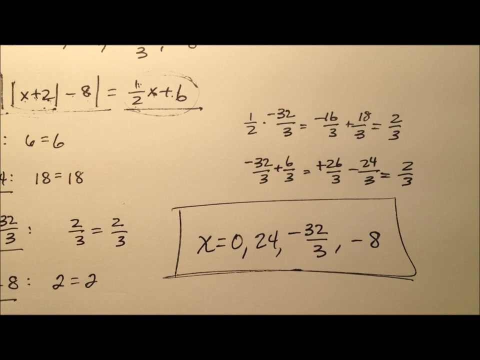 So all four of these answers work, and so we have four solutions to this original equation. They're going to be: x equals 0,, 24, negative 32 thirds and negative 8.. And again going back to our original equation, we had this nested: absolute: